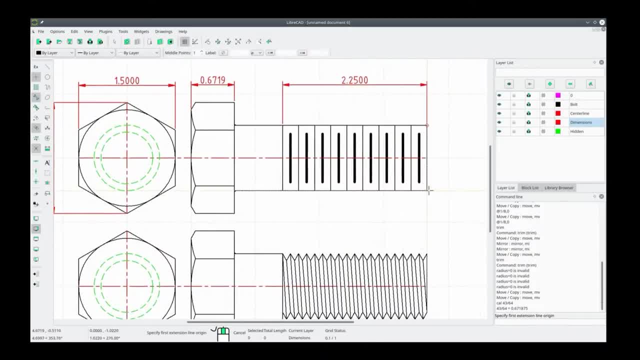 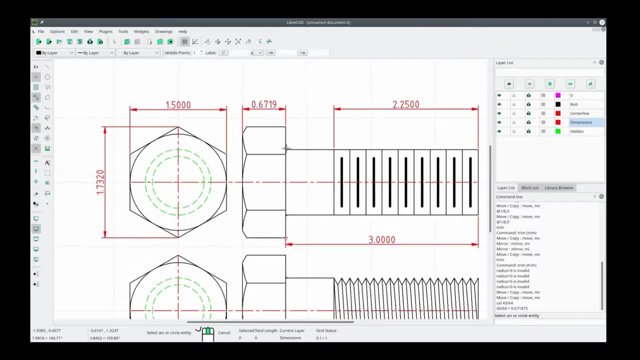 and it even can be used to do interior design sketches, mechanical parts, schematics and diagrams, and it supports different kinds of formats like DFX, SVG and PDF. The tools and features are easy to use and it can be used by students, hobbyists and even professionals. 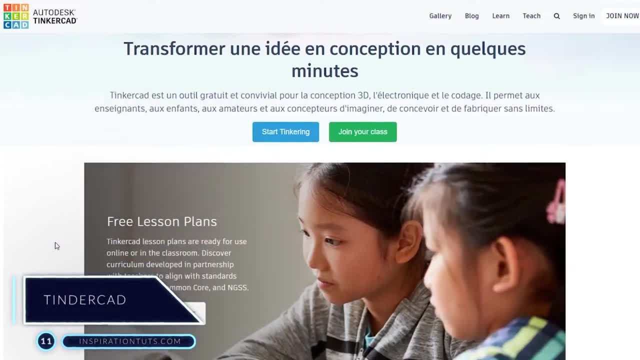 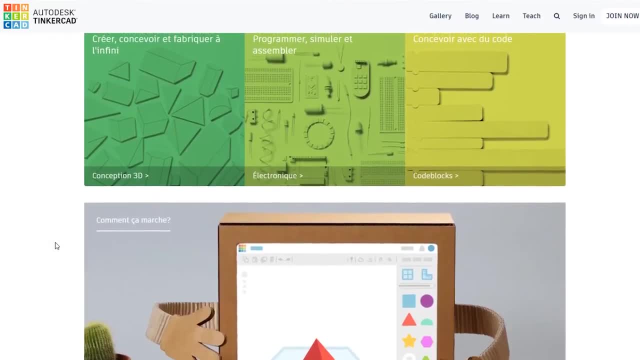 Tinkercad. This software is used a lot by students and professionals because it helps them start designing simple objects and make progress when making complicated objects. It can also be used in 3D printing, jewelry design, interior design, toys, prototypes and so on. 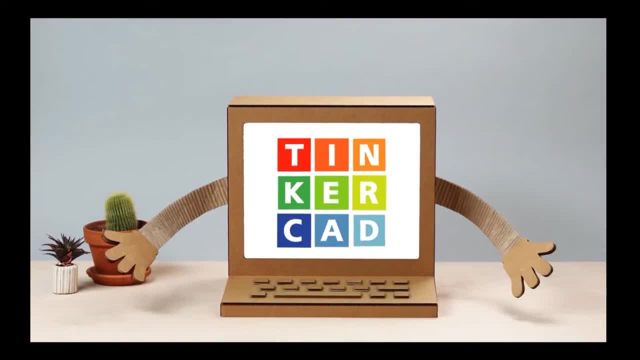 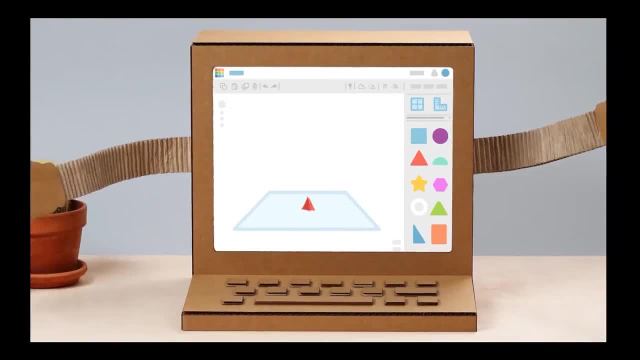 The software offers a lot of good features, like intuitive interface, some design tools and modeling tools, in addition to code blocks. You can save your work in the cloud. In addition to that, the software is very light and it doesn't require a lot of space or a strong computer. 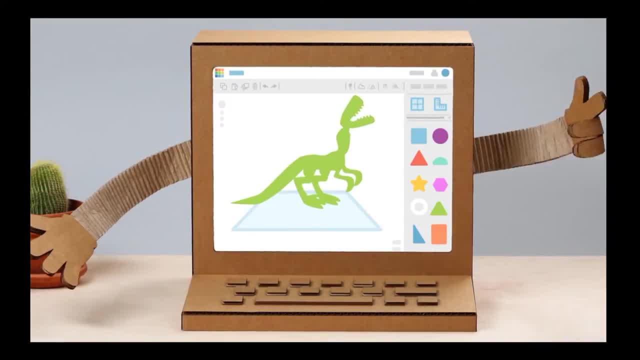 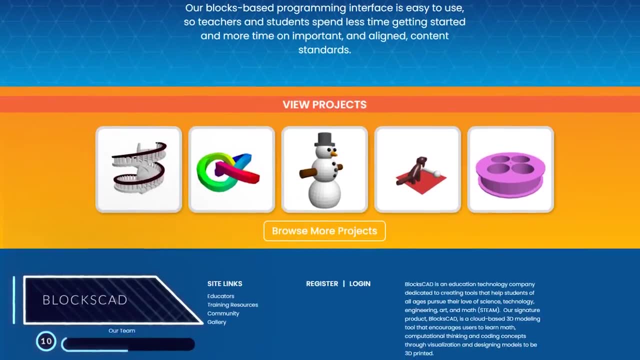 And the best part is it is completely free. Number 10, BlocksCAD. It is a web-based application to do 3D modeling and animation. The 3D designs that the software generates can be used in webinars, presentations, websites and even social marketing. 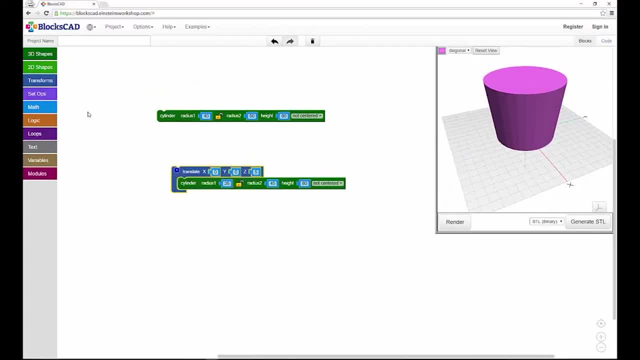 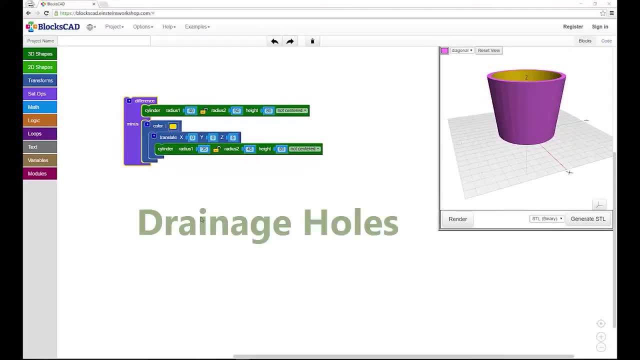 This web application is used a lot by startups and agencies. It offers a lot of good features like 3D modeling using drag and drop coding and so on. It is also very similar to OpenSCAD: It uses the same coding to create and combine geometric objects. 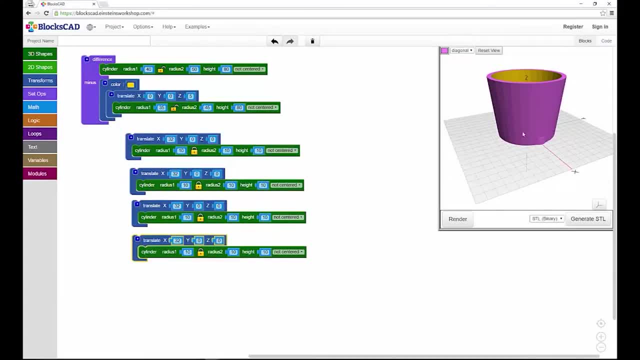 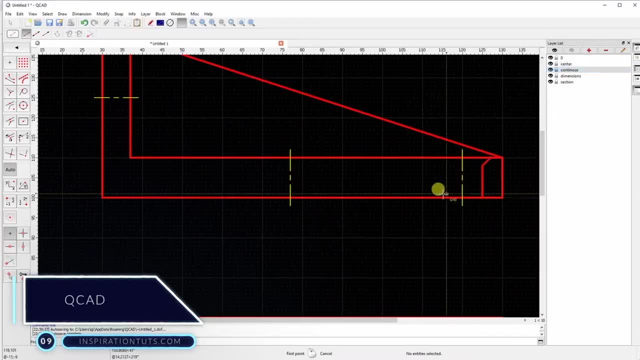 This web application costs 149 US dollars per year. This web application costs 149 US dollars per year. Number 9,: QCAD. This is a free and open-source CAD software. It was made to do 3D drafting, but it has good tools for creating complex technical details. 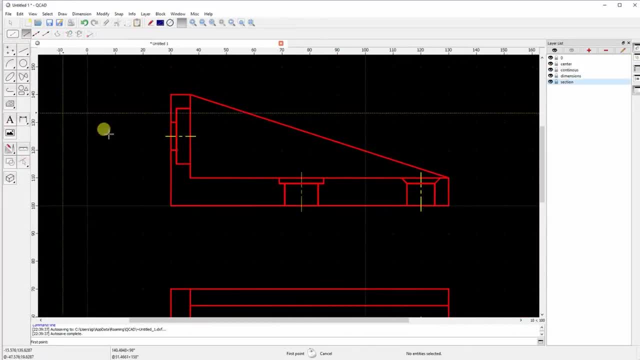 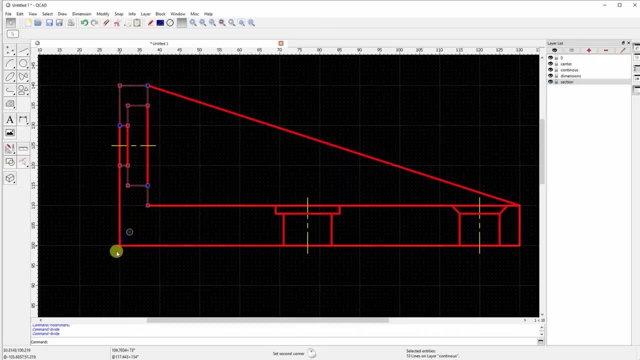 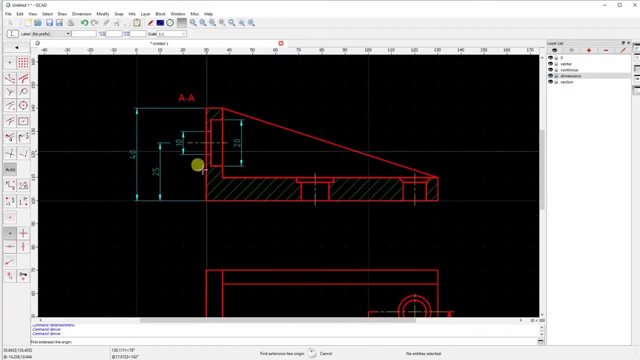 It is especially great for graphic design. You can precisely set all the measurements and the dimensions relative to your design or mechanical piece. It is compatible with all CAD software because you can open QCAD files in other CAD software. You can also use metric and imperial system, and the software needs a little bit of training. 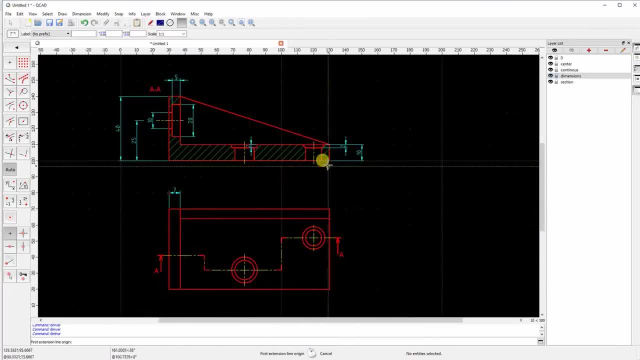 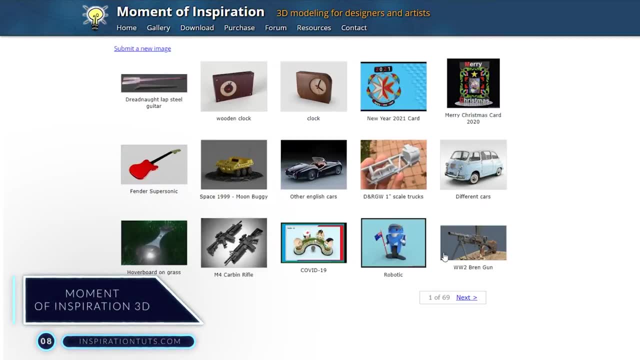 can use it, especially for beginners and students who are not familiar with CAD software. Number eight: Moment of Inspiration 3D. It is an intuitive 3D modeling software with powerful tools and anyone can use it, even if you are a beginner or if you are not a designer, Because the interface 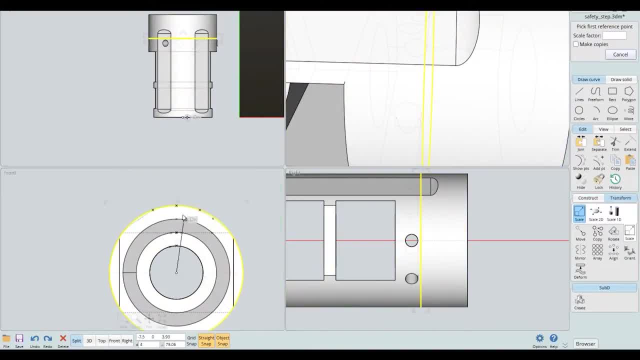 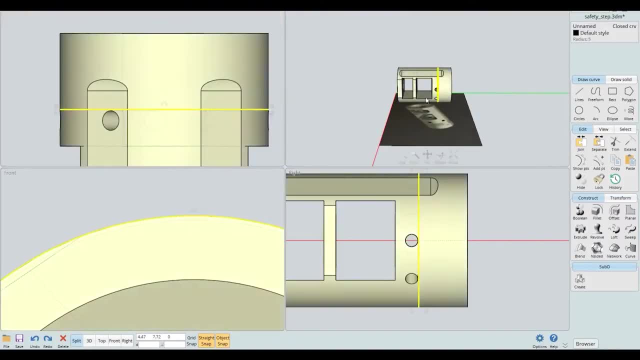 is so simple and straightforward and it is one of the low-cost solutions in the CAD family. It can also work perfectly to create mechanical pieces, solid and hard surface models. Additionally, you can use the software on a tablet with a pen easily, which allows you more freedom in the 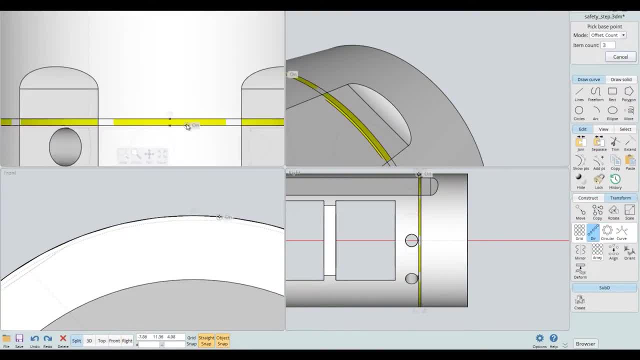 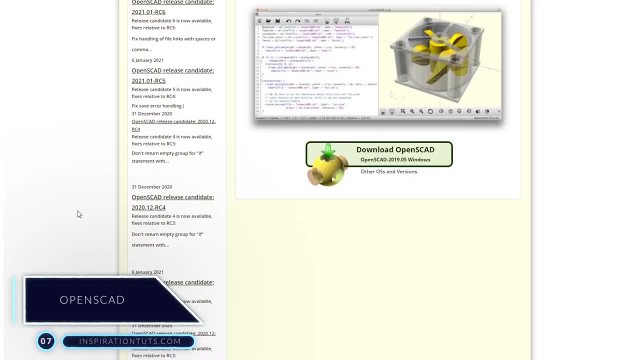 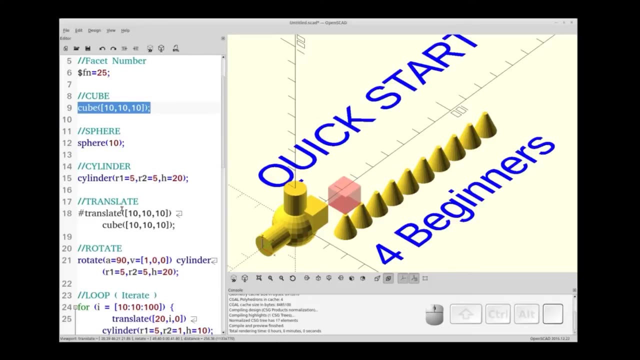 design process. You can get this software for 260 US dollars and it is available for Windows and Mac. Number seven OpenSCAD. It is a great software to create solids in 3D. It can also be used to create parametric geometric objects. The workflow of this software actually depends on your experience. 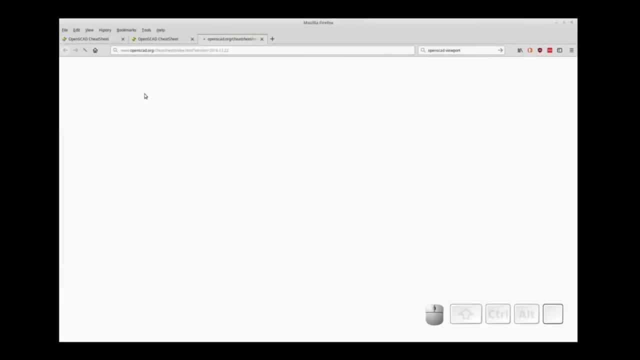 whether you are a beginner or a professional, Working on parametric object designs help you adjust them individually. If you are a beginner or a professional, you can use this software to in the future to suit different needs. You can also use coding to set up all the parametric parts. 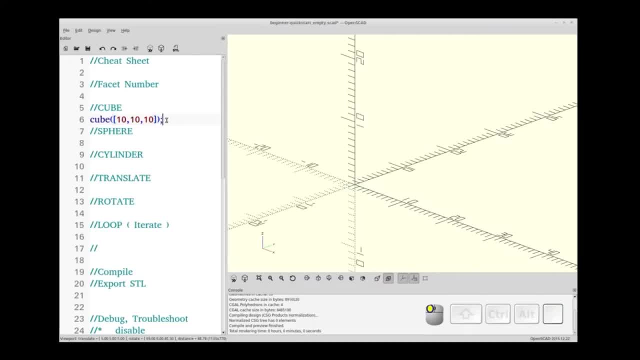 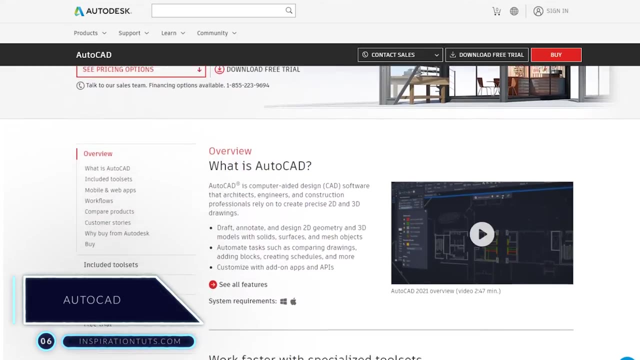 relative to your objects. It also offers GIT configuration management, which is very great and a helpful option. Overall, OpenSCAD is a great software to program in multiple languages and can be used in 3D printing as well. Number six, AutoCAD. It is one of the first products released by Autodesk and it is a great 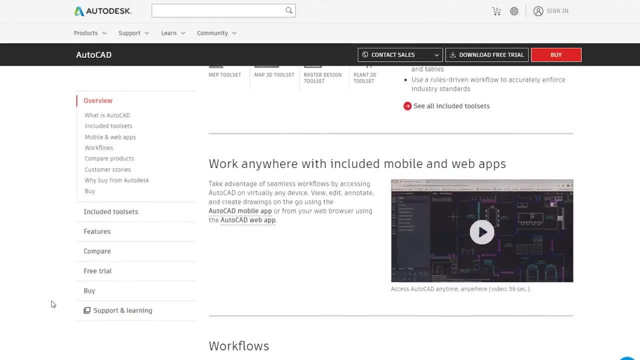 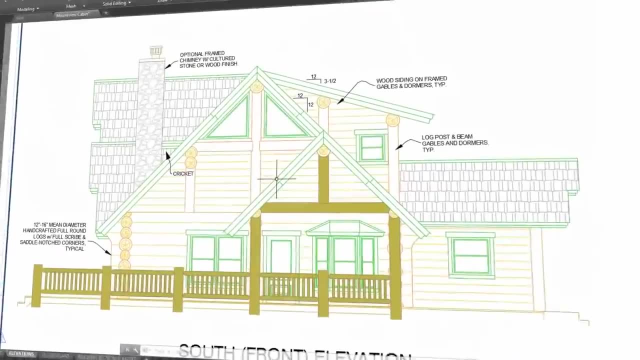 start for beginners and students, since it has an easy interface and the tools and the commands are direct and easy to use. AutoCAD is commonly used in 2D drafting in different fields like architecture, mechanical, electrical parts and so on. The 3D part of AutoCAD can be a little bit. 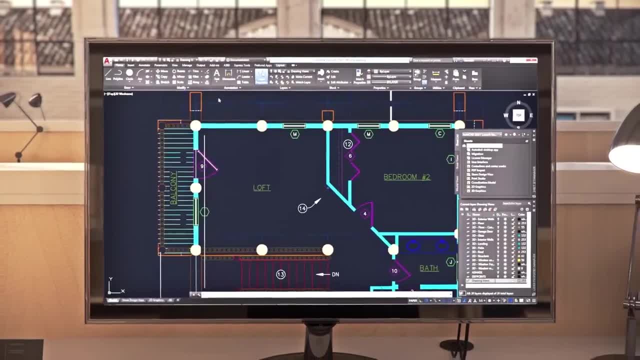 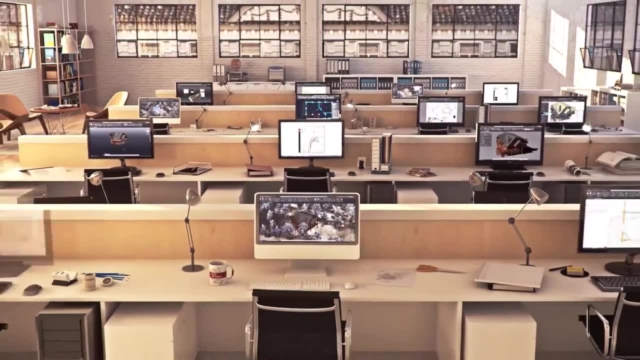 complicated and it doesn't offer a lot of features in terms of 3D compared to the other 3D software, but learning AutoCAD will open for you the way to learn more software more easily. It is available on Windows and Mac and, later on, a web app called AutoCAD 360.. 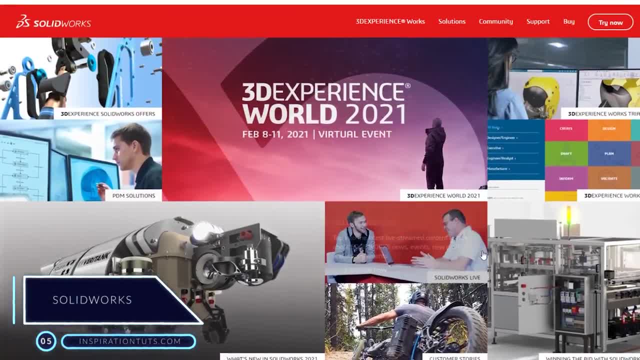 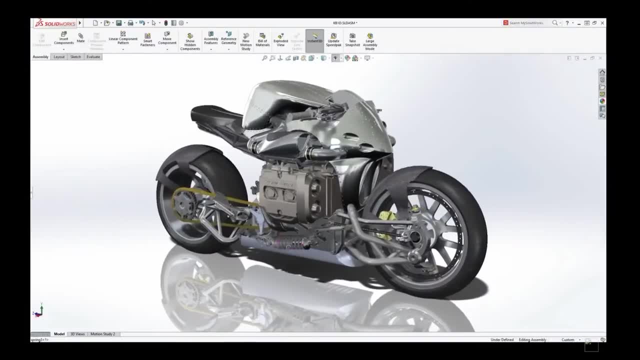 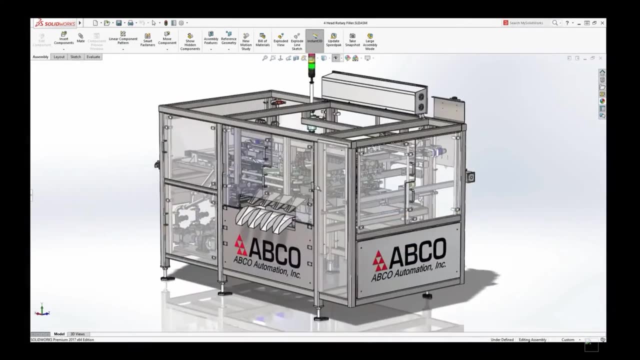 Number five: Solidworks. Solidworks is made essentially to do complex 3D designs, such as mechanical and electrical pieces, because it has great tools for creating complex details. The software can help you create all kinds of objects, assemblies and presentations of products to clients. in the end, It also offers 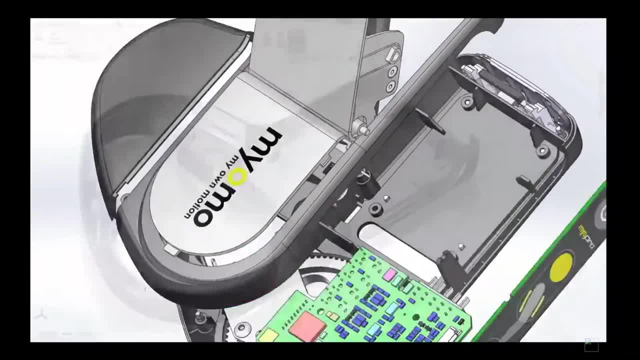 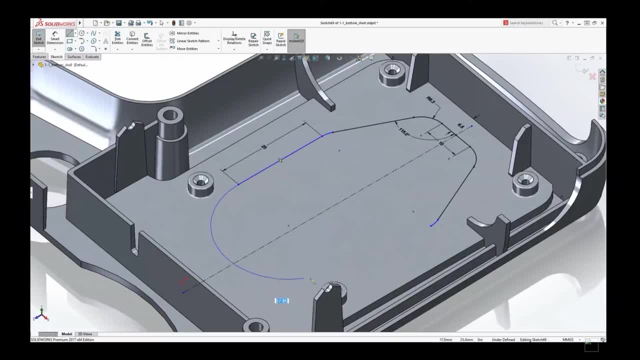 all the necessary basic tools to create simple products, like the ability to change area weight dimensions, and it has advanced and precise drawing tools that you can use to create complex models and assemblies. Solidworks is known for being one of the simplest, most efficient and most efficient software to use among professional CAD software. 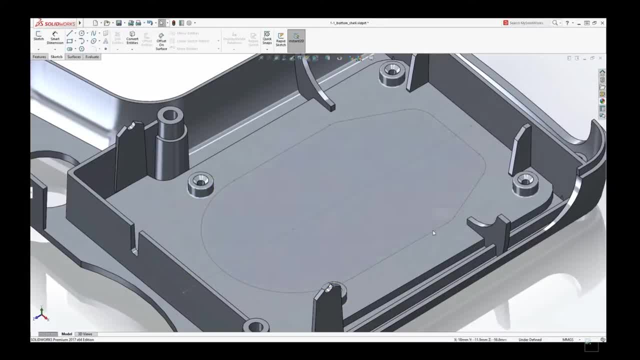 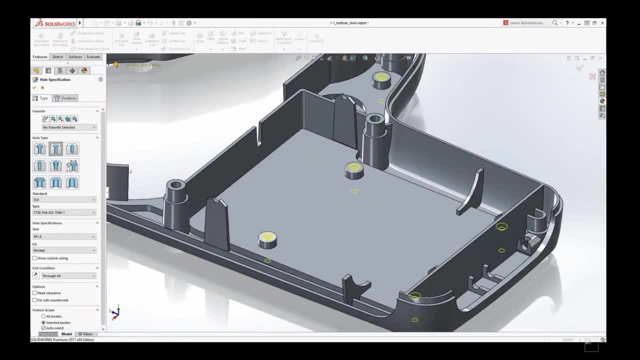 but it is a little bit more limited in terms of using curves. For instance, when it comes to card design, it can be hard using it, especially when creating curved surfaces. Overall, it has great and easy tools, since its users pay very close attention to details, especially when it comes. 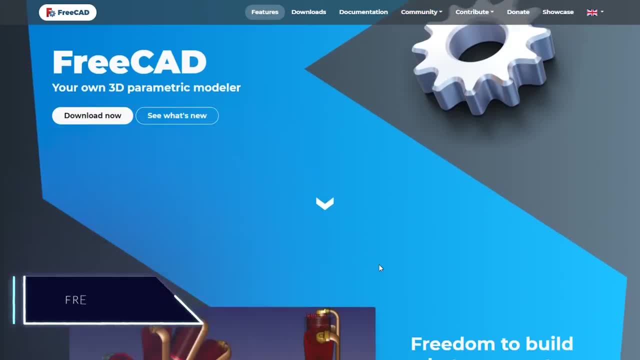 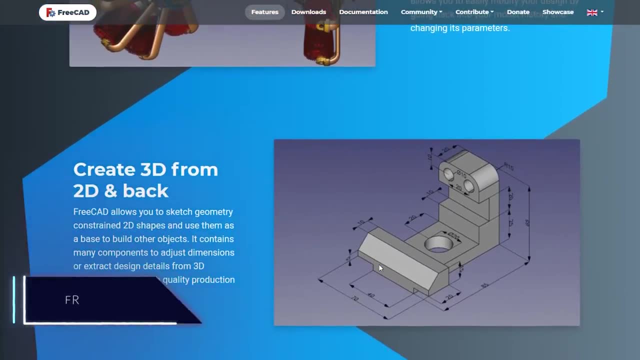 to technical drawings and 3D modeling. Number four: FreeCAD. FreeCAD is a modeling software made essentially to design complex objects, especially mechanical stuff. It can be considered simple and easy to use, especially for basic designs. It can also be used in different 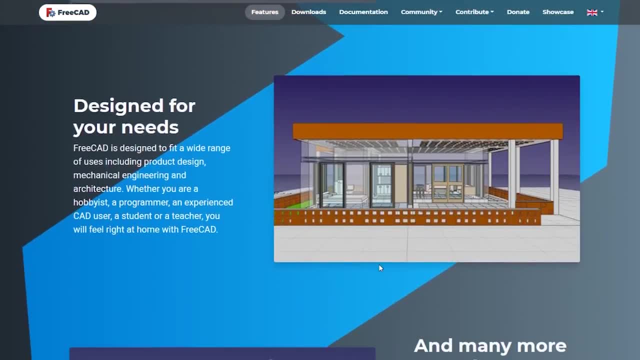 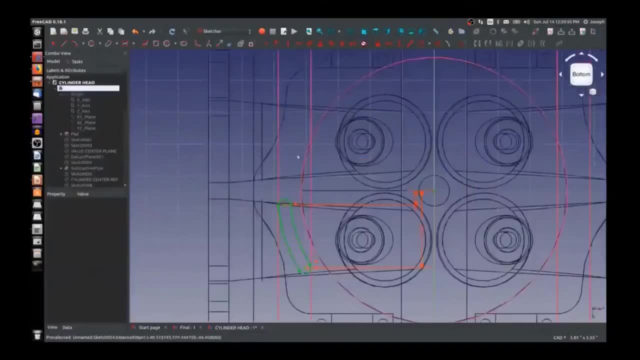 industrial fields. in addition to architecture, You can also use it to design complex objects and even to do rendering. In addition to that, it has a great parametric workflow where you can regenerate your models by changing some variable values. You can also use this software to design. 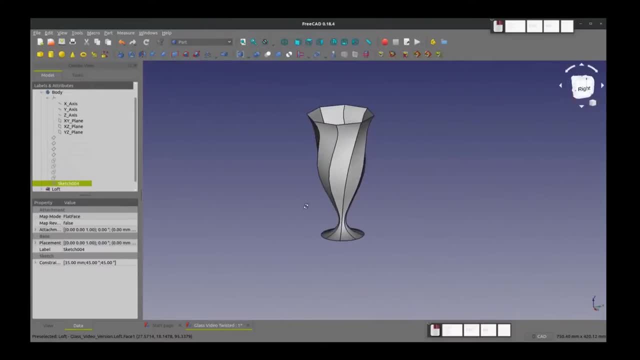 from scratch or to do reverse engineering. The software offers great features that can be found even in paid software. Besides that, FreeCAD is open source and it is very easy to use. FreeCAD is a very simple software that can be used to design complex objects and even to do rendering. 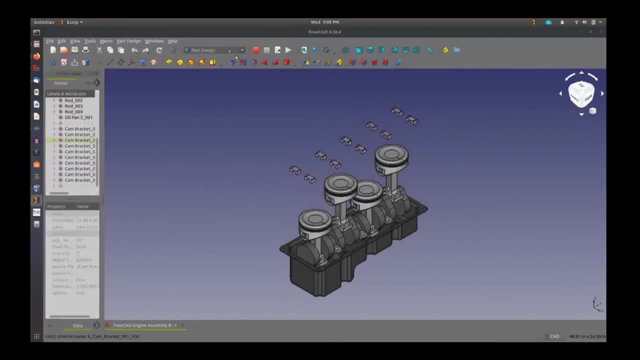 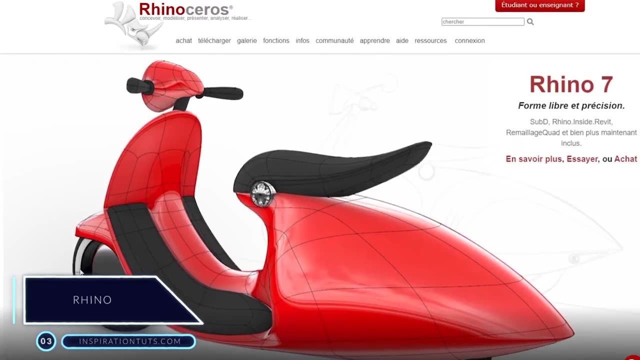 It also has GUI mode and it can run on Windows and Linux. Number three, Rhinoceros 3D. This is a great modeling software that can be used in different fields. It can be used to model houses, furniture and objects such as cars, jewelry and so on. 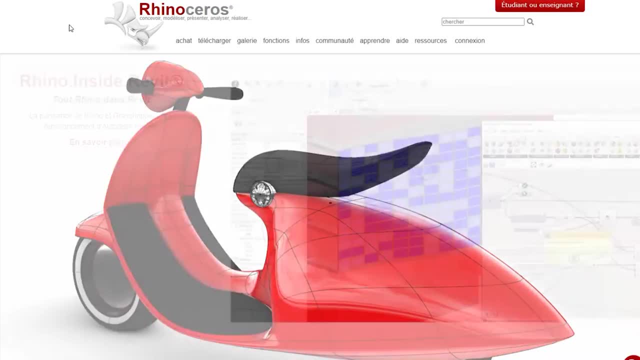 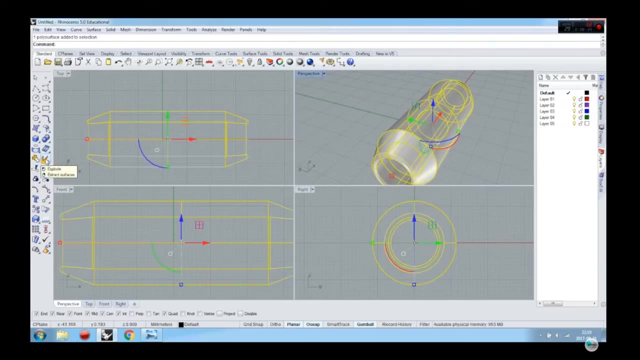 It is relatively easy to use because its interface is clear, simple, with many tools and features. Its tools allow you to have a high precision when working on complex 3D models like cars and jewelry, And over time, the workflow of the software will be fast because you'll be able to get used to it. 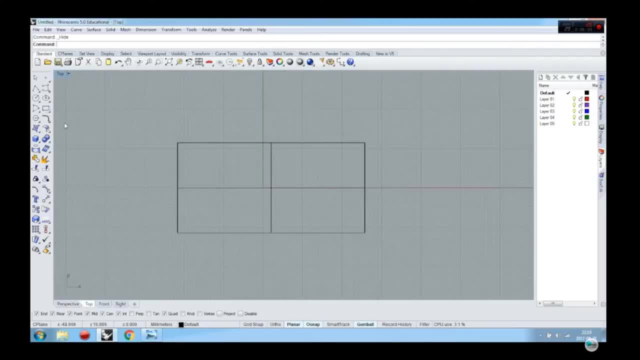 especially when you start using shortcuts and hotkeys. Overall, it can be used by beginners for small projects or by professionals when working on complex ones, And the good thing about Rhino is that you can download plugins and customize the software and have a smooth workflow. 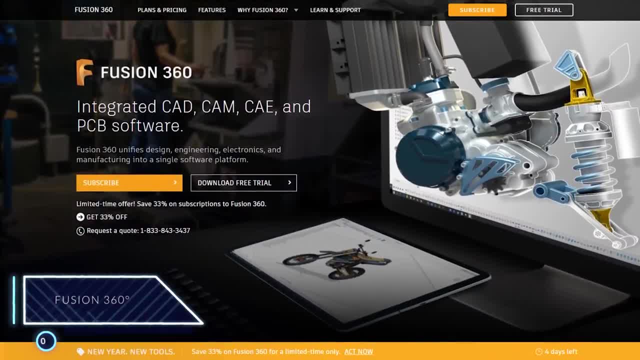 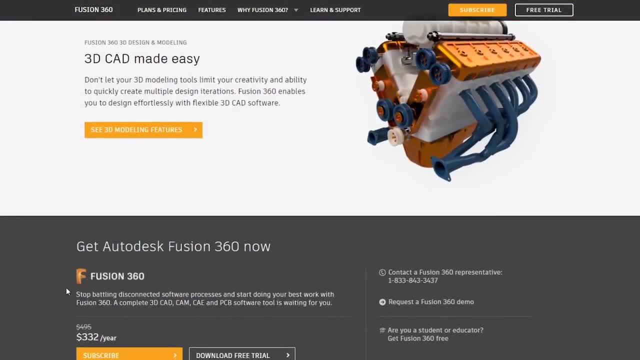 and better results. Number two: Fusion 360.. Fusion 360 was made specifically to do mechanical and technical object design. Fusion 360 was designed specifically to do mechanical and technical object design. It also offers you the possibility to model artistic 3D objects and it can also be used to do 3D.